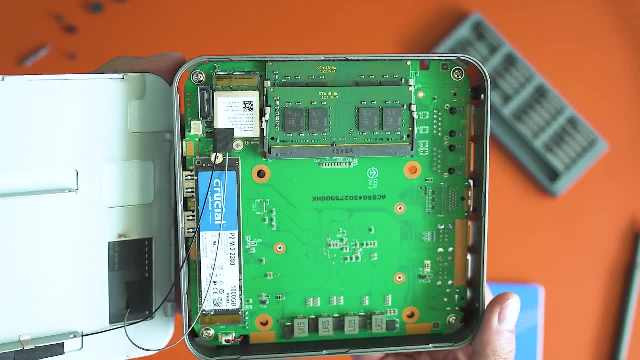 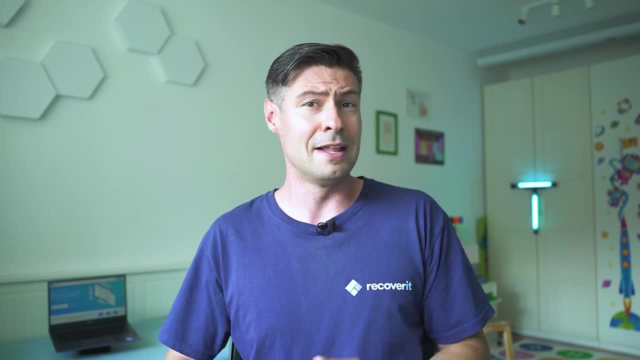 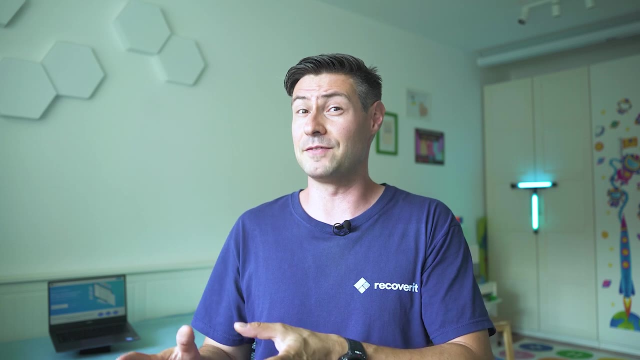 flash storage, micro SD card and many, many others. In most cases, the file system allows us to manipulate these files in the way we want, as long as it is supported by the file system, like copying, leaving, renaming, deleting, etc. etc. So, in short, this would be the part of the 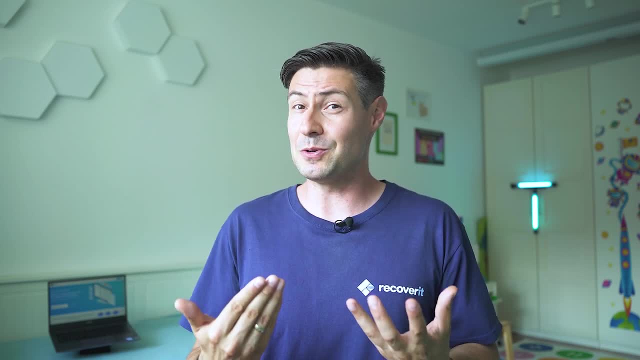 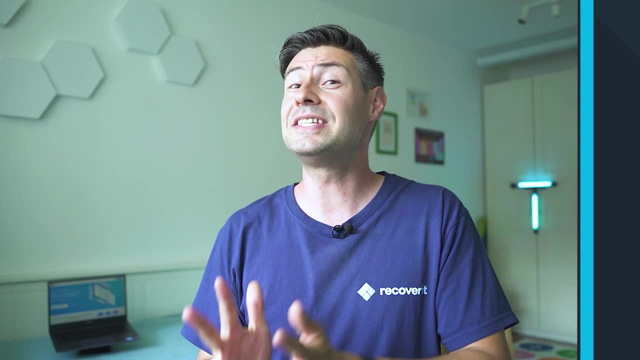 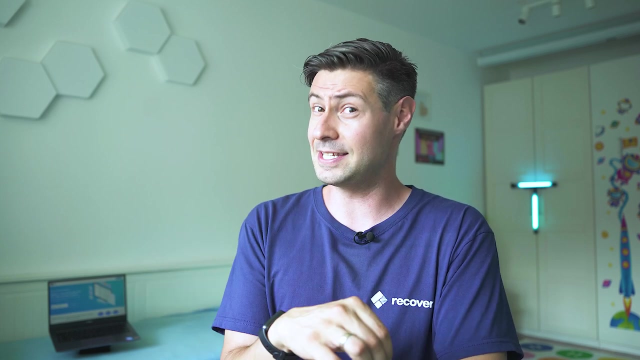 operating system which is allowing us to handle and manage the files which are stored on the drives. This leads us to the next important characteristic, and that would be the type of the file system. It's a fact that most different operating systems support different variety of 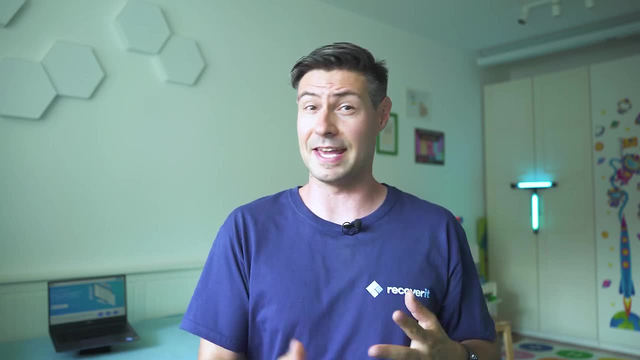 file systems and could be that, for instance, if you use an Apple device and they have their own proprietary CPU with many different access to these files, they have their own properties based on the size of the wall and they do not have to have multiple files in this case. 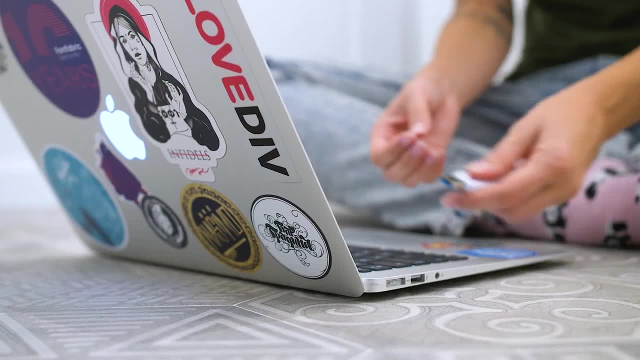 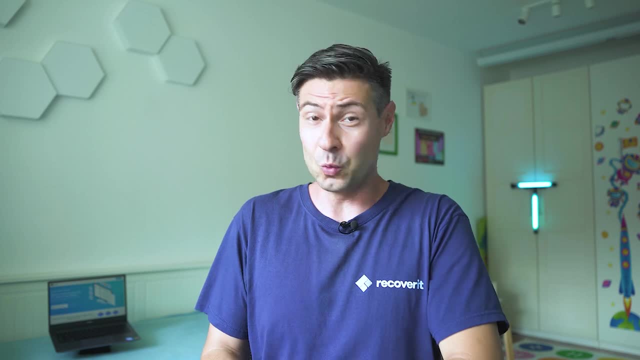 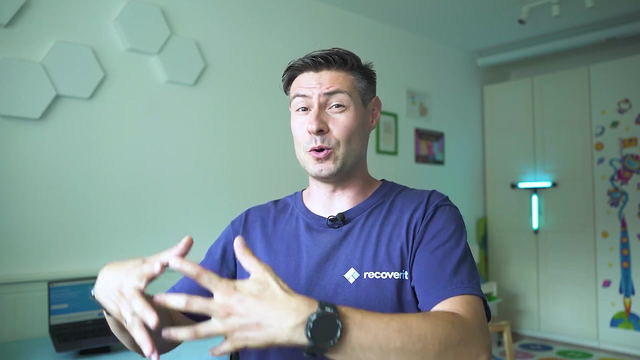 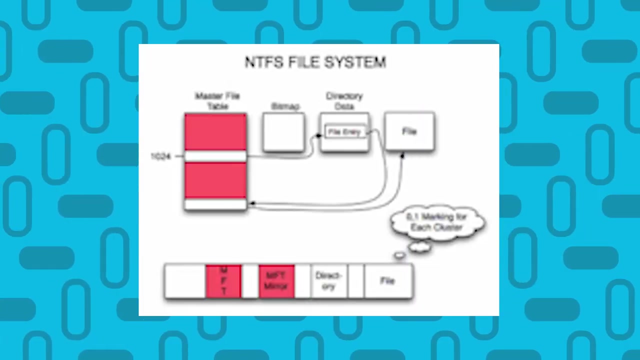 proprietary Apple file system. it wouldn't be accessible or readable on a Windows workstation. So how all of that really works. Well, you could consider the file system as an index for all the data which is stored on a storage device. The file system specifies the naming structure and the rules to name different files. 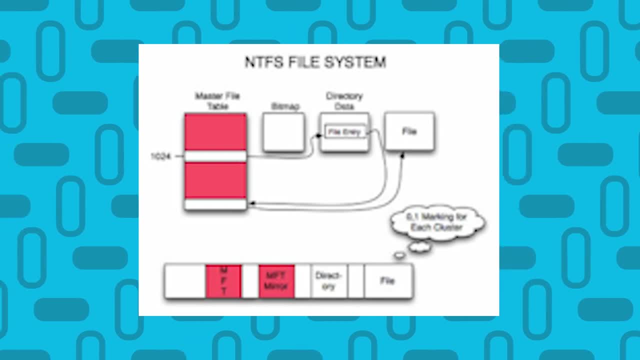 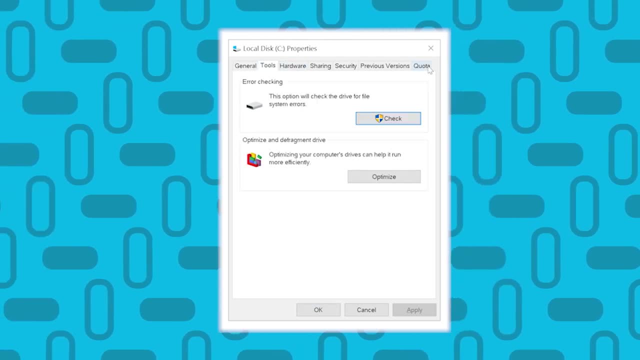 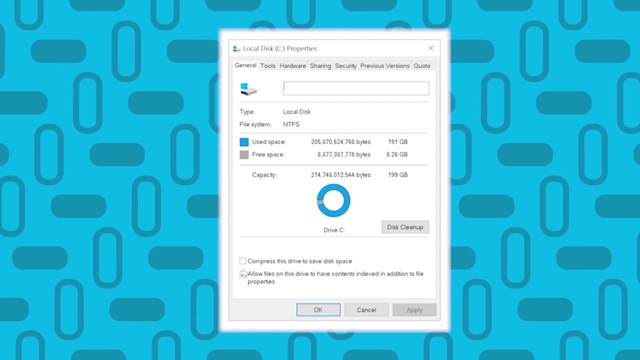 Some file structures are case sensitive in nature, which means that you can't use uppercase characters to the file name. The file system also defines the character length of a file. While naming the files, you can't go beyond the specified character limit. otherwise the file system automatically triggers an error message. 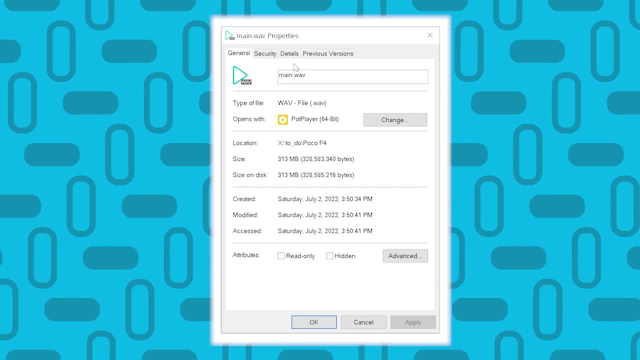 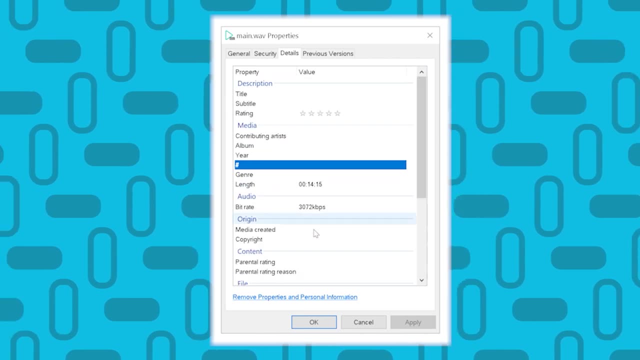 Apart from the basic information, the file system also holds advanced details, such as the size of the file, its attributes and its target location. All these details are stored in the file, The metadata, which is a separate block on the storage device that your system uses to fetch data from the file. 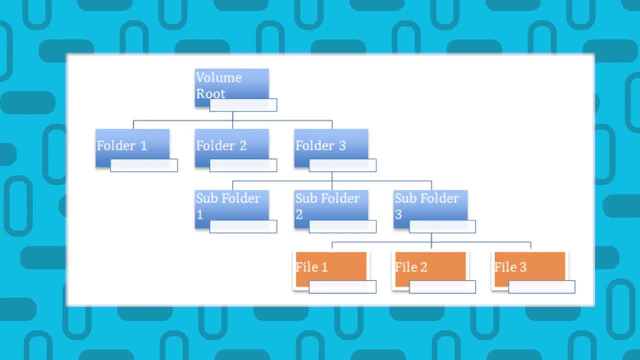 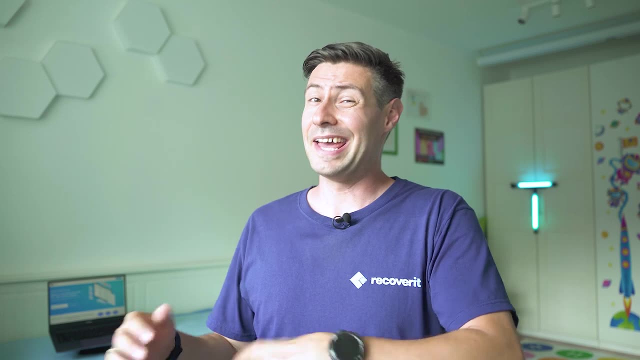 This metadata also stores a directory error key to pinpoint the exact location of a particular file on the storage device. Now coming to the types of the file systems and, as we mentioned a bit earlier, certain operating systems have access to certain file system types. 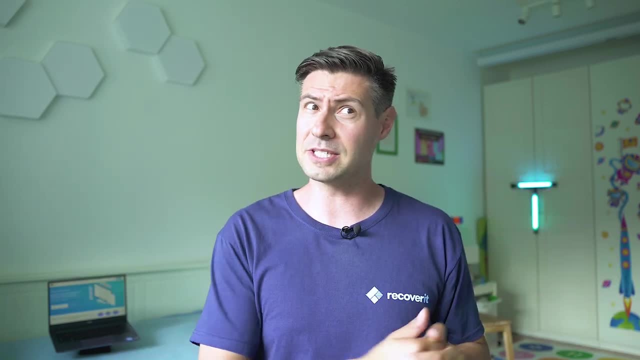 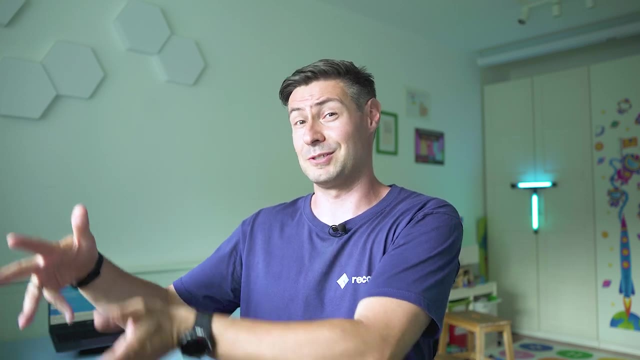 Some OSes could support a wider variety of file systems, some not really. I guess we're going to start with the most popular one And that's related to the Microsoft Windows operating system. It's called FAT, so popular FAT file system. 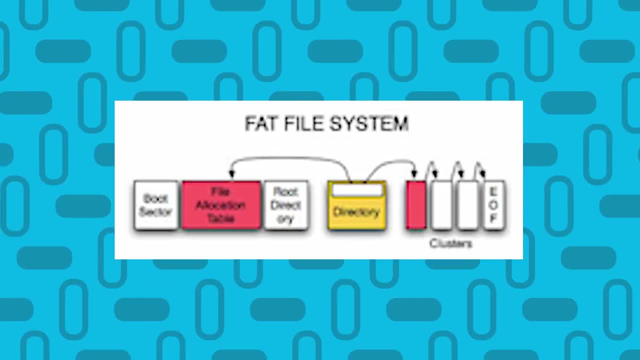 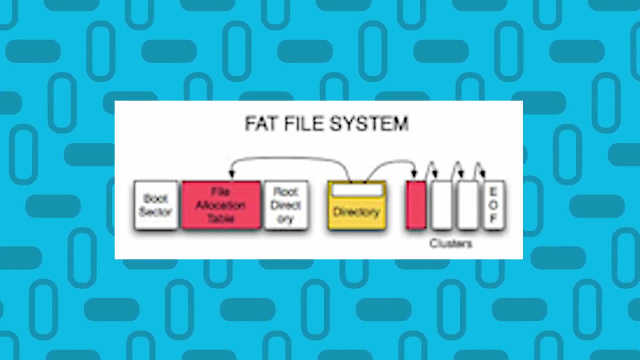 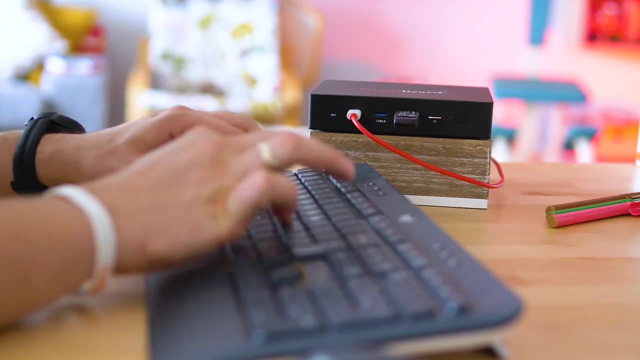 It's probably one of the oldest file systems, which are supported by multiple operating systems, including Windows. FAT stands for File Allocation Table. In many situations, a file is broken down into multiple sections that are scattered across the hard drive of a system. The FAT file system is responsible for keeping a track of these systems. 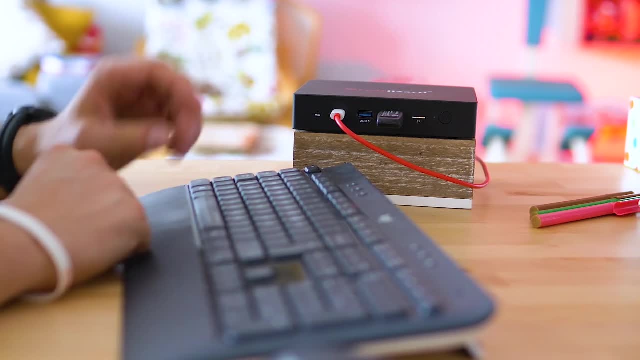 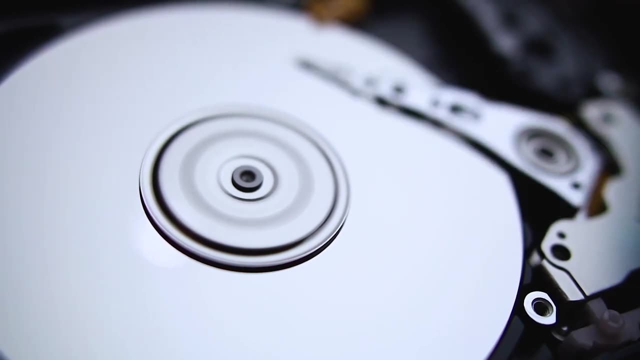 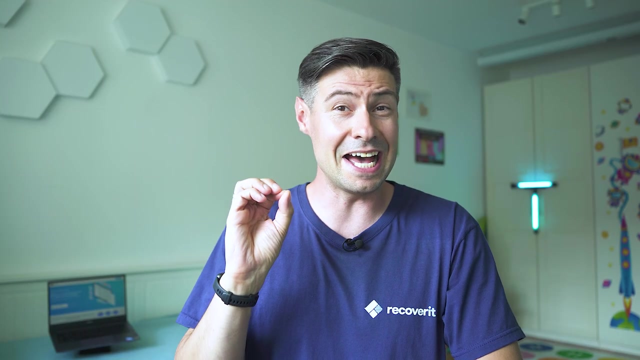 It's also responsible for making it easier for the system to fetch the data when requested. Ideally, the FAT file system supports up to 8 characters, and the name should always begin with an alphanumeric character. Okay, going further with FAT32, or FAT32,. it's the advanced version of the original FAT file system, so it's an improvement. And it's mostly targeted at customers running Windows 2000 and older, meaning that you can still find it well-supported with some computers that are being utilizing newer and fresher versions of Windows. It's very suitable for devices coming from a size of 512 megabytes up to 2 terabytes. 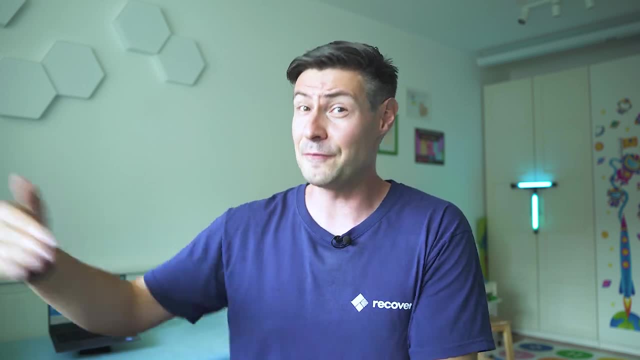 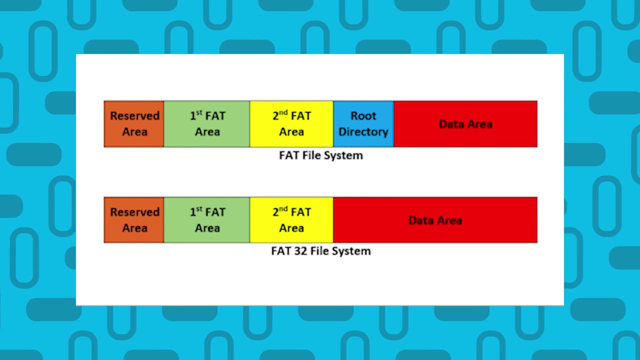 and they do support a much greater amount of files to be stored. FAT32 makes disk utilization more effective, as it can access files more rapidly across different storage devices. Continuing with NTFS- and I remember it's something that was presented for the first time- 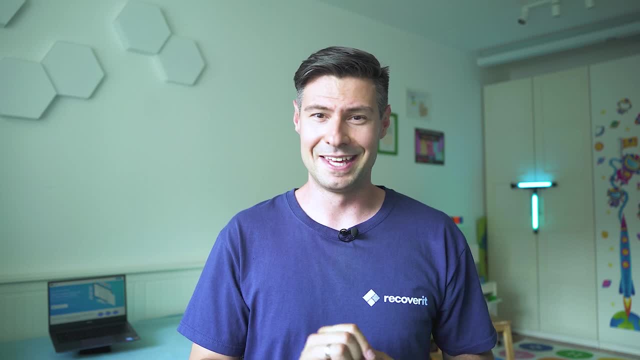 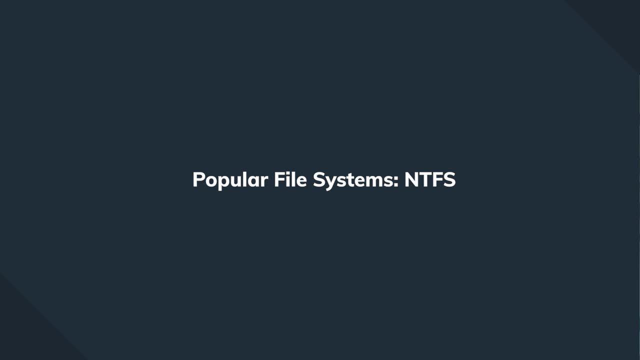 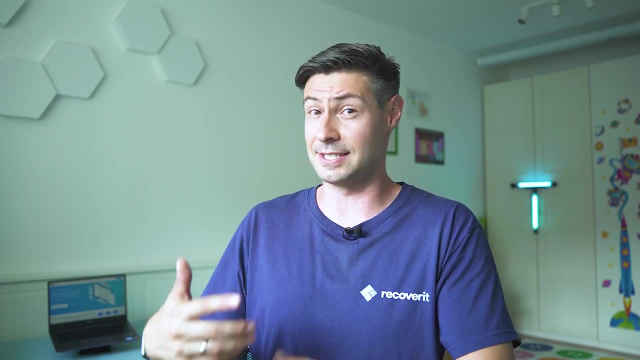 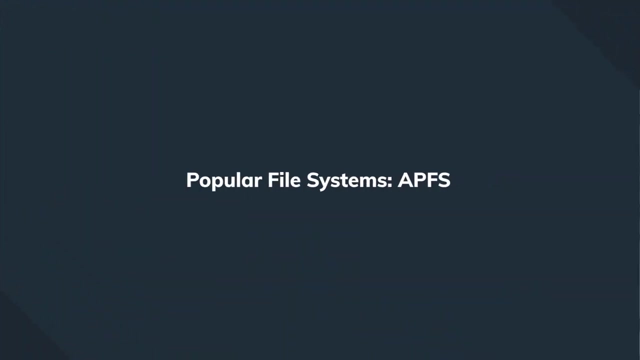 but going backwards was a no-go Anyhow. so with NTFS, everything is a lot more advanced and the file system is no longer case-sensitive, meaning that, as a user, you have the liberty to name the files the way you want. Next, APFS. 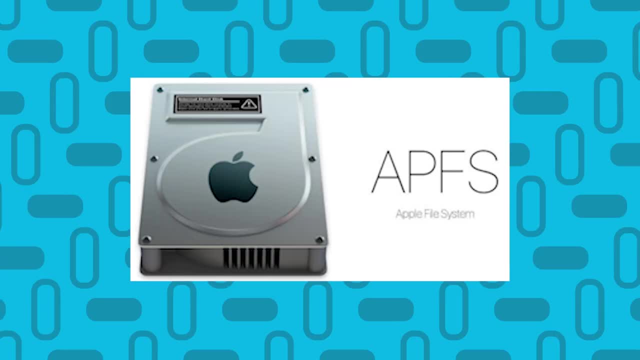 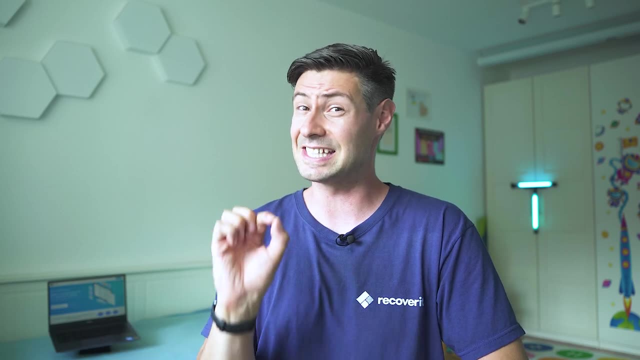 That's the Apple File System. It's something that the company has been using for a long time and the company has developed back in 2016, in order to strengthen its position and to also improve the performance on its various devices. But the thing is it's only supported on iDevices- on Macbooks, iPhone, iPod, etc. 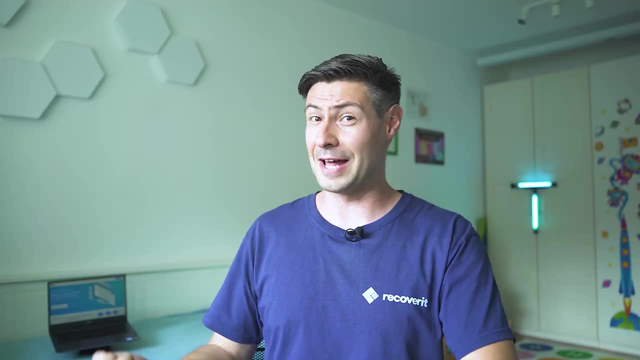 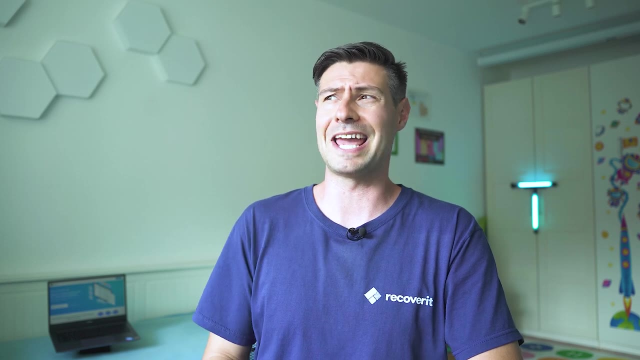 On Macbooks, iPhone, iPad, etc. Thing is, if you format a flash drive into APFS, It's only going to be accessible by operating systems which are capable of reading APFS. so understand iOS or Mac OS. Therefore, in order to read and write data,